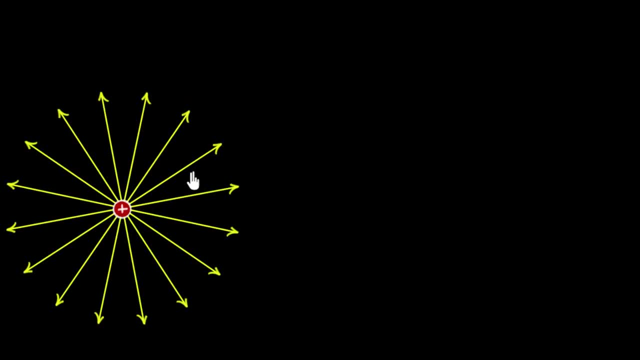 We've learned how to visualize electric field by drawing field lines. In this video, let's explore how to visualize electric potentials And the way to do that, or at least one way of doing that- is by drawing something called equipotential surfaces. 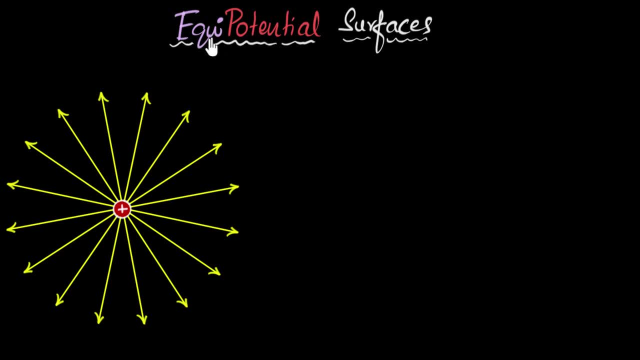 So what exactly are these? Well, as the name suggests, these are surfaces, and these are three-dimensional surfaces over which the potential at every point is equal: Equipotential surfaces. Let me give you an example. So if we come over here, 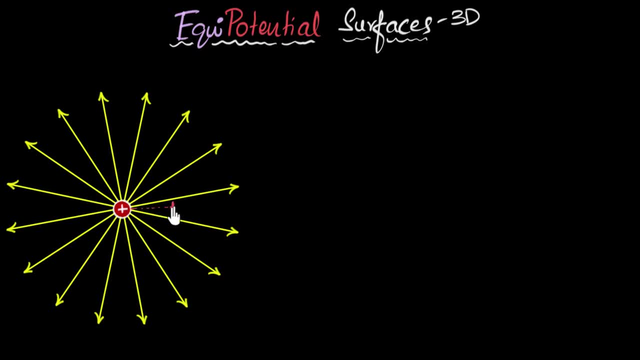 let's say, from this charge I go about two centimeters far away over here. There will be some potential at that point. Let's call that as 10 volt. Let's imagine that to be 10 volt. Now, if I went two centimeters over here from the charge, 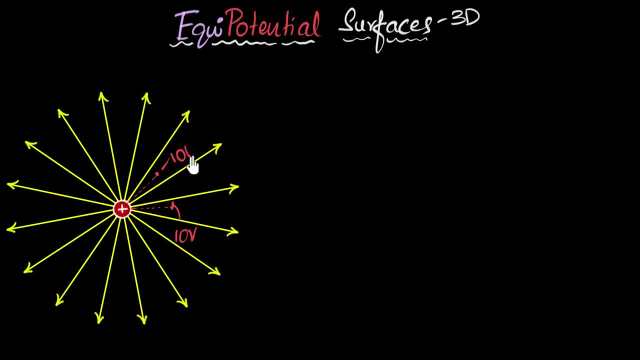 what would the potential there? It should also be 10 volts. What about two centimeters from here? That should also be 10 volt. In fact, I could draw a circle of two centimeters, and two centimeters is just an example. okay. 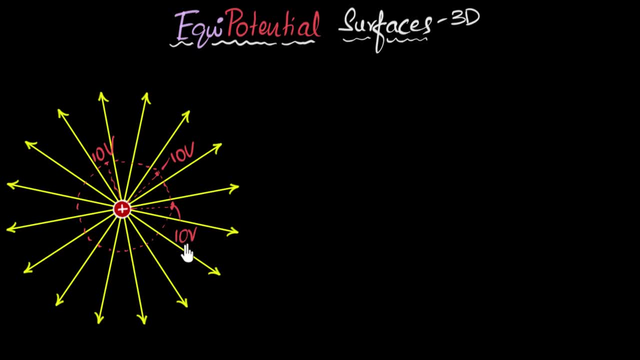 And everywhere on that circle the potential would be equal 10 volt. So that circle would be an equipotential surface And since it's a three-dimensional, you have to imagine this actually is not a circle, but it's a sphere. 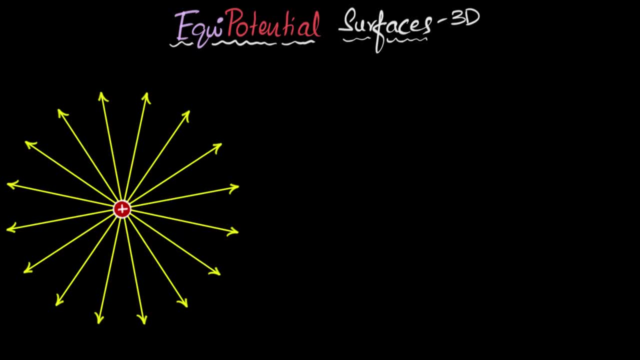 So let me just draw that nicely, So I could draw a sphere. let's see here it is a sphere. You have to imagine this is a three-dimensional sphere where on every point of it the potential is 10 volt equal. 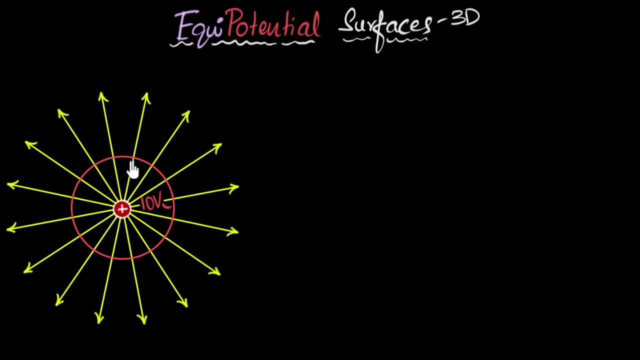 And so this would be my 10 volt equipotential surface. Can I draw more? Of course, If I go a little farther away, maybe two and a half or three centimeters far away, I would draw another sphere. that would be another equipotential surface. 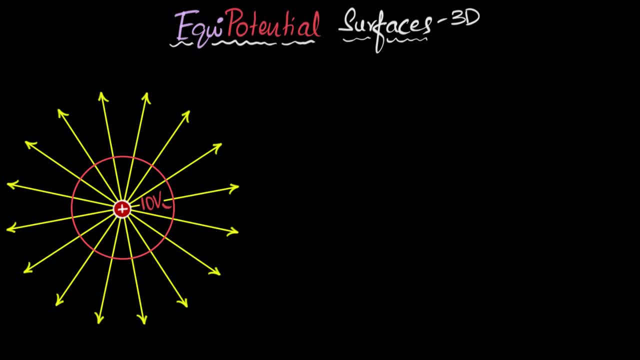 Let me draw that If I go farther away, the potential will decrease, right? So let's say this is another equipotential surface. Why is this equipotential? Because on every point of it the potential is equal, And it's equal to seven volt. 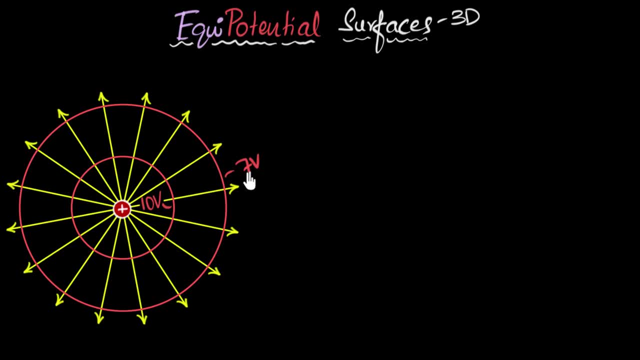 Can I draw more? Yes, more spheres. Every sphere you draw will be an equipotential surface. In fact, if I go a little farther away and I draw another one, I might get a nine volt equipotential surface. If I go a little farther away and I draw another one. 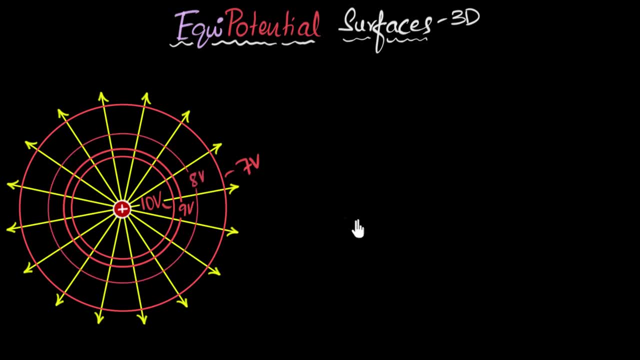 I might get an eight volt equipotential surface and so on and so forth. Now, before we continue, you may immediately notice that the surfaces are closer here and they're going farther and farther away. Why is that? Well, it's got something to do with the strength. 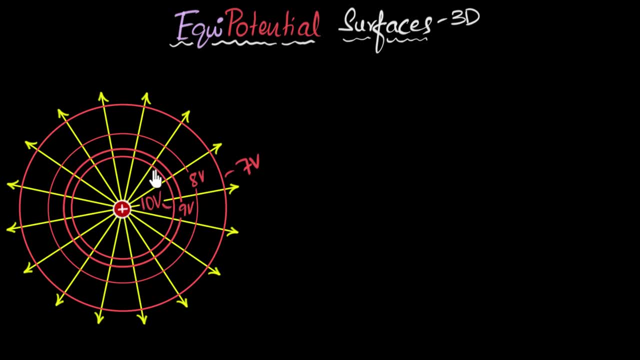 of the electric field Close to the charge. the field is very strong, and that's where the equipotential surfaces will be closer to each other. As we go far away from the charge, the field weakens, and so the surfaces go farther and farther away. 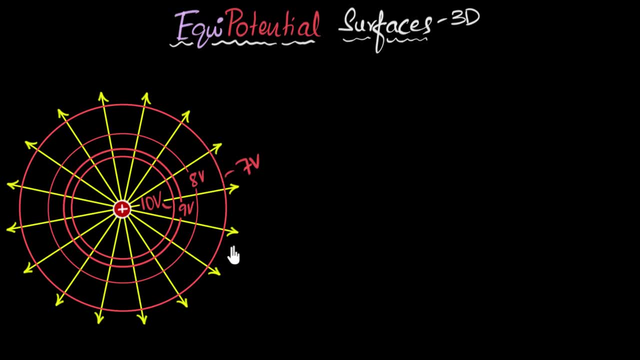 from each other, But why? Why is it that if the field becomes weaker, the equipotential surfaces go farther away? Can you pause and think a little bit about this? All right, here's how I like to think about it. Consider a tiny test charge kept over here. 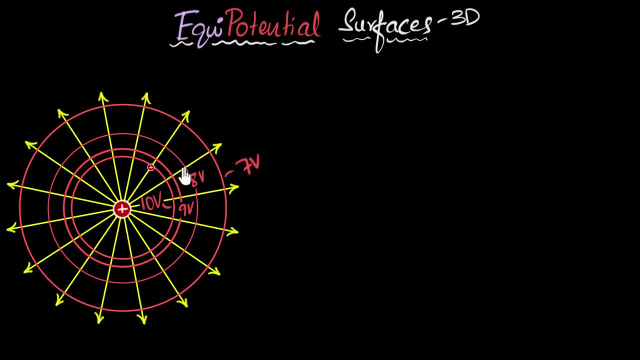 on the 10 volt equipotential surface. What will happen if I let go of it? Well, the electric field will push it and it'll accelerate and it'll move from this equipotential to another, the nine volt equipotential. 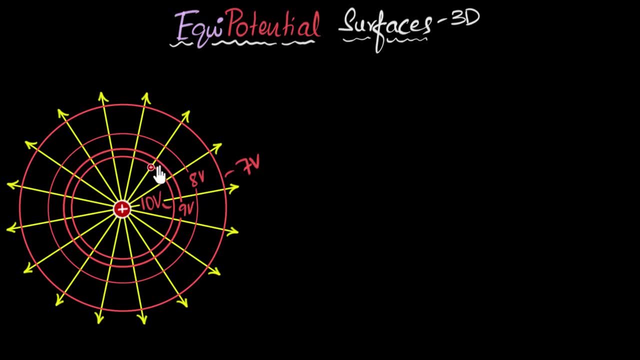 Now, because the force over here is very strong, because you are in a strong electric field region, it will accelerate very quickly, it will gain kinetic energy very quickly and, as a result, it will lose. it will lose potential energy very quickly. 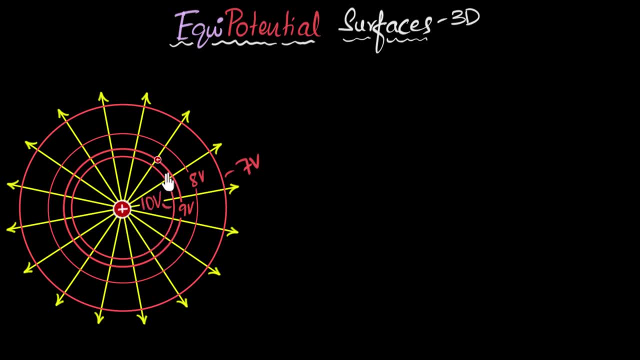 And it's for that reason in a very short distance, it would have reached from 10 volt to nine volt equipotential surface. However, what would happen if I were to keep that same test charge over here? Well, now the field is very weak. 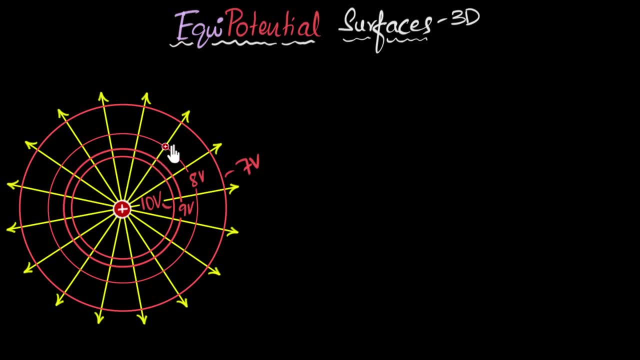 or weaker compared to here, and so the force acting on it is very weak, and so it'll accelerate slowly, And so it's gonna take more distance for it to pick up the kinetic energy, and so it's gonna lose potential energy more slowly and, as a result, 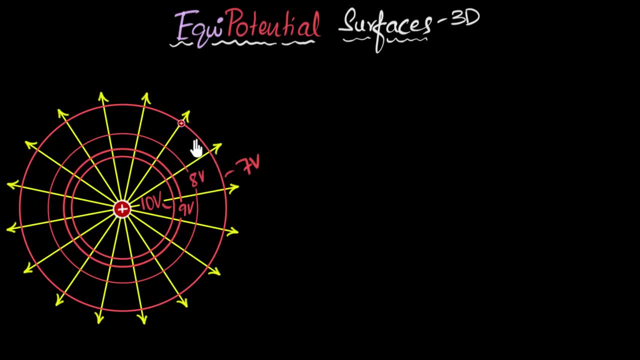 it's gonna take a longer distance before it reaches. it loses one volt now, And so what do you think will happen for the six volt equipotential? It'll take even larger distance to reach six volt, and so it'll be even farther away. 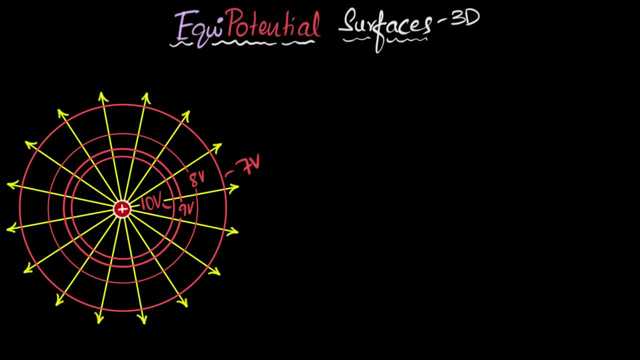 Does that make sense? It's kind of like if you take a ball and drop it on, say, Jupiter, where the gravitational field is very strong, then it'll accelerate very quickly and so it'll gain kinetic energy very quickly, so it'll lose potential energy very quickly. 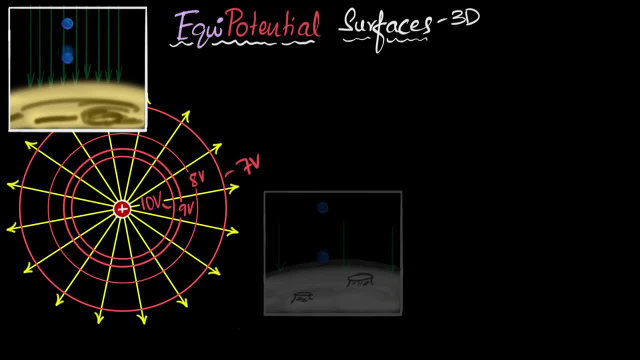 But, on the other hand, if you were to drop that same bowling ball on, say, Moon, well, because the gravitational field is very weak, it's gonna accelerate very slowly, gain kinetic energy very slowly and so therefore lose potential energy very slowly. 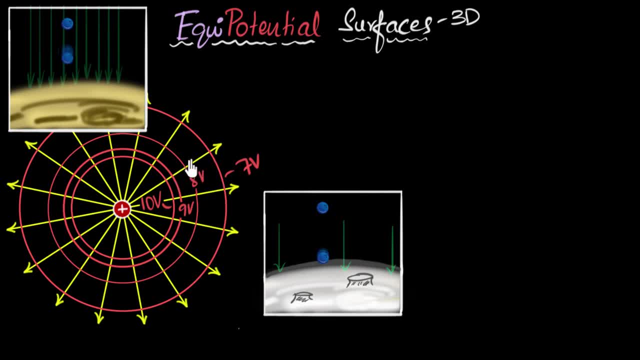 So, weaker field in weaker fields, you lose potential very slowly, and so the potential surfaces are farther away. All right, let's take another example, and I want you to take a shot at drawing equipotential surfaces. Let's say we have a long, long, long, long, long, long long. 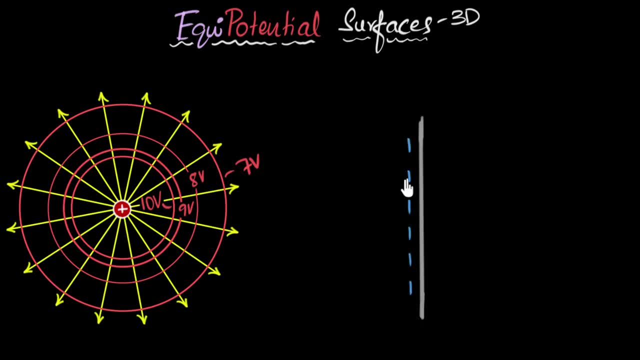 infinitely long sheet of charging, big sheet of charge which has, let's say, negative charge. Then we know we've seen before. it produces a uniform electric field. Can you think of what the equipotential surfaces here would look like? 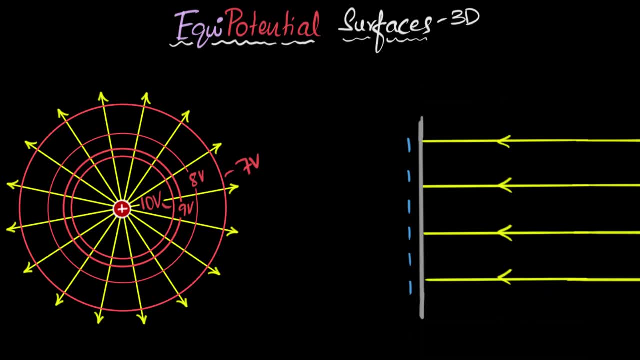 Can you try drawing a few equipotential surfaces over here? Pause the video and think about this. Use the same approach as we did over here. All right, just like over here, let me go at some distance, say about two centimeters from this sheet. 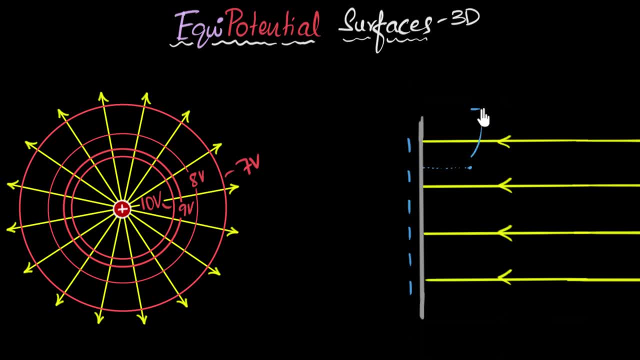 It'll have some potential because it's a negative charge. maybe there's some- I don't know- negative 10 volt potential. Now, if I go two centimeters from here, I should get exactly the same potential as here, And the same would be the case over here as well. 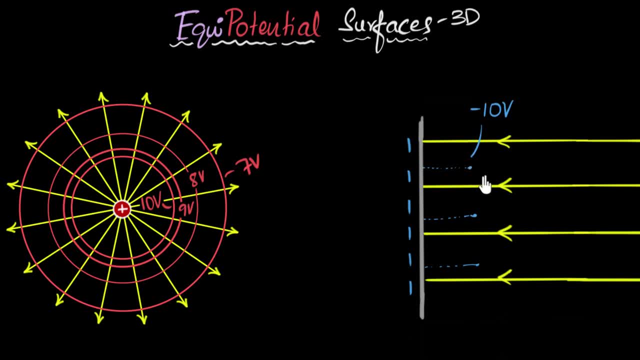 Ooh, that means I can draw, connect all these lines, and if I do that now, my equipotential surface would look somewhat like this. So this would be my minus 10 volt equipotential surface. I can draw another if I go a little bit farther away. 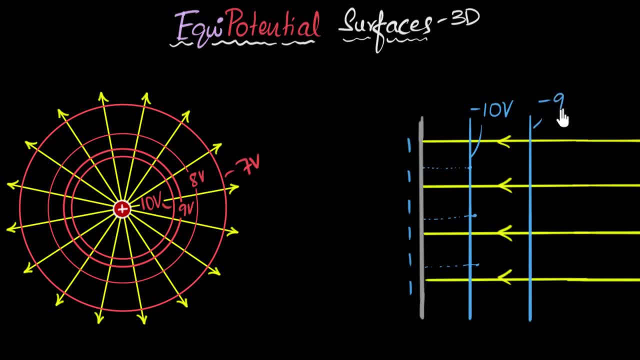 maybe I'll get another, let's say minus nine volt equipotential surface. If I go farther away, maybe I'll get another minus eight volt equipotential surface, and so on and so forth. Over here I hope you agree that the equipotential surfaces will be equidistant. 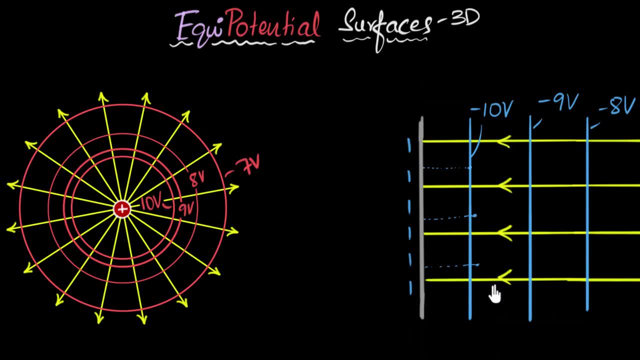 because the field lines are all, the electric field is uniform And again, just to reiterate, this is not a line, this is a surface. so you have to imagine this in three dimensions. I'll help you visualize that If you could see this in three dimensions. 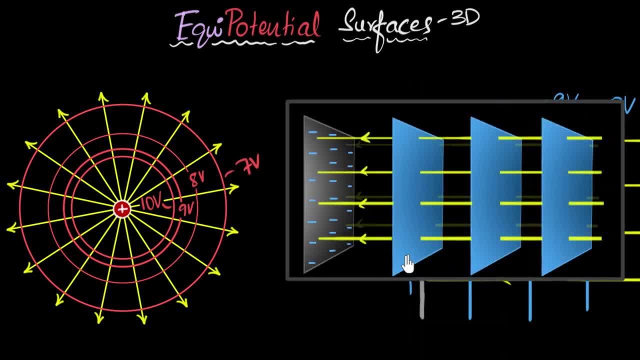 So if you look at them in 3D, you can now see that now the equipotential surfaces are plane surfaces. So over here we got spheres, over here we're getting plane surfaces, All right, but here's a question. These were simple cases. 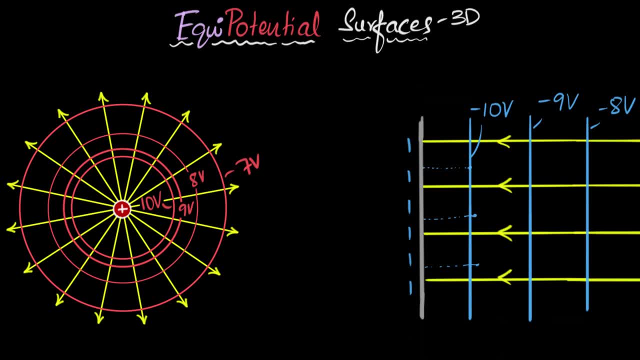 What if we have to draw equipotential surfaces in general? What if I have some random electric field line due to some complicated network of charges, Something like that? I don't know, just randomly drawing? How would we draw equipotential surfaces? 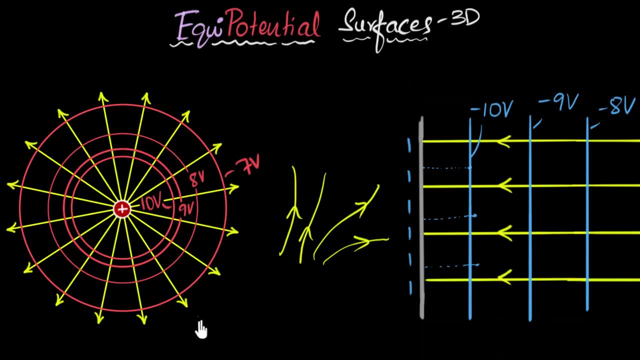 then We may not be able to use the same approach like here, but what we can try to do is see if there is some geometrical relationship between electric field lines and equipotential surfaces. So let's come over here. Can we see any relationship between these field lines? 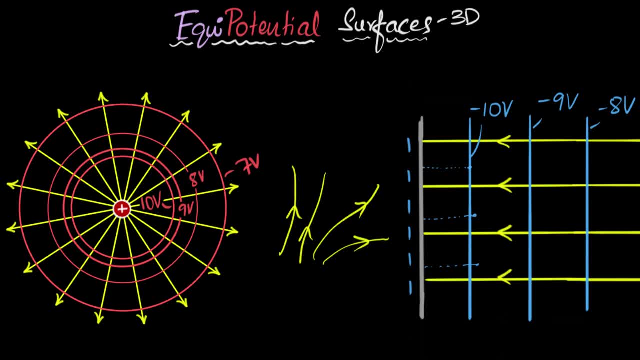 and the potential surfaces. If you look very closely, you can see that these equipotential surfaces are perpendicular to the field lines. And that makes sense, right, Because in general over here the field lines are forming the radius and the radii are always perpendicular. 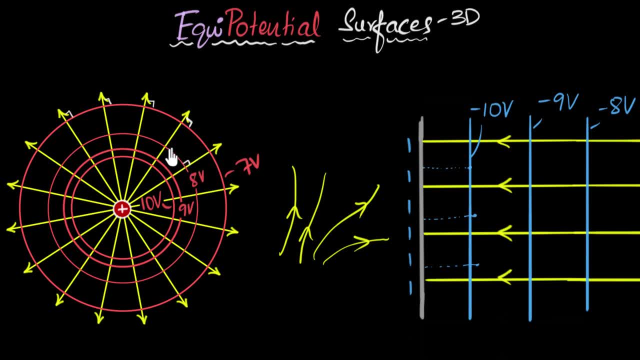 to the spheres or circles. So over here we are seeing that the two are perpendicular to each other. hmm, Let's look at over here. Hey, here also we are seeing that the field lines are perpendicular to the equipotential surfaces. 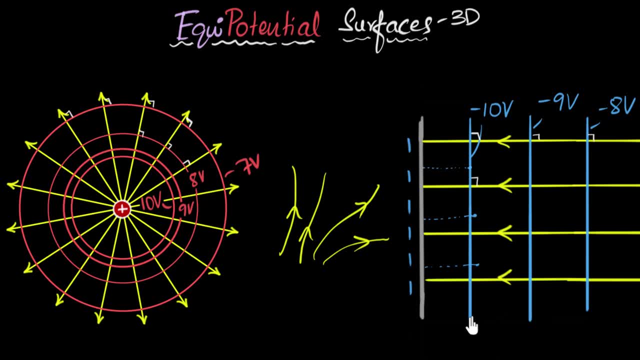 Hmm, interesting. So can we say that this is true in general, That equipotential surfaces and field lines must always be perpendicular to each other? We can't just say that using two examples. we could say that might be a coincidence. 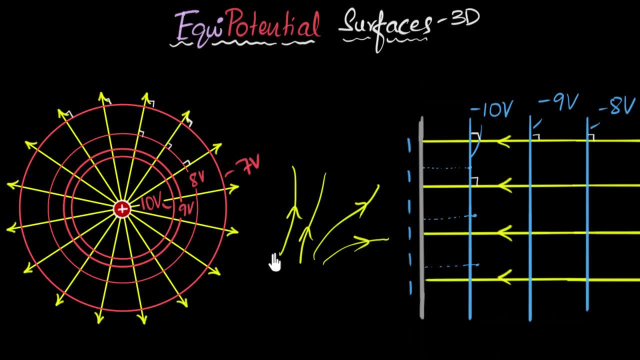 So is this true in general? Well, if you and I were in the same room, maybe we would have an interesting dialogue over here, but I don't want to take too much time and I'll go ahead and tell you that turns out. 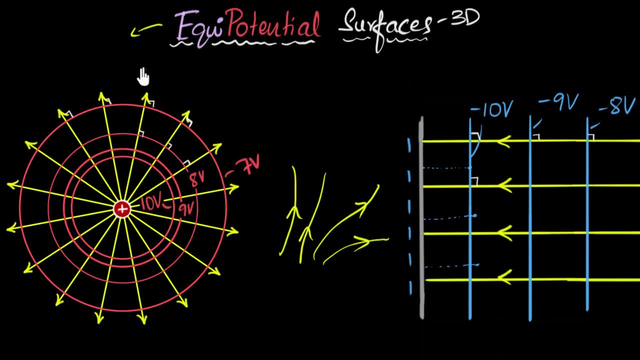 that this is true in general. So let me just write that down. Equipotential surfaces are always, always perpendicular to electric field lines. I can just say perpendicular to field or field lines, Always, Regardless of how complex the field lines are. 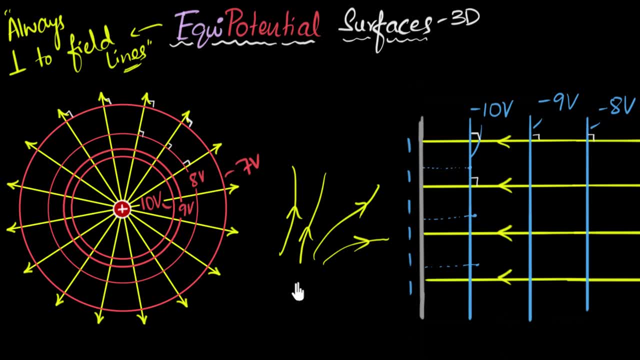 And again, the final question for us in this video is why this is true, And I want you to again pause and ponder upon this. This is a deep question, but I'll give you one clue. Think in terms of contradiction. What would happen if the equipotential surfaces? 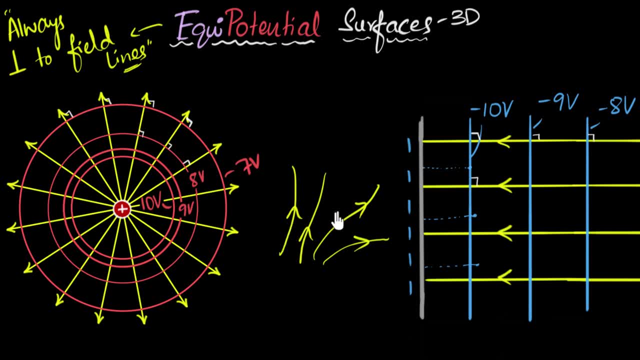 were not perpendicular to the field lines. What gets broken? Think a little bit about that. Like I said, it's a deep question. Don't expect it to get right away, and it's okay if you don't get it right away. 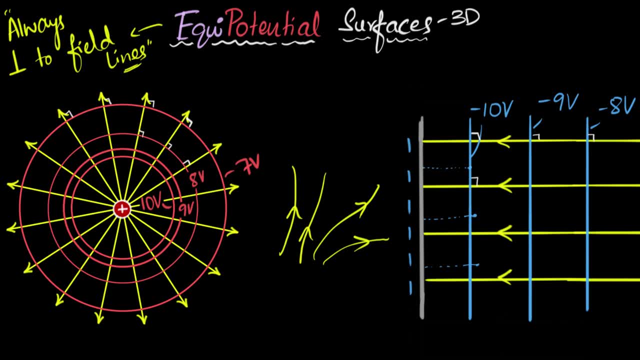 but the idea is just to think a little bit about it before we go forward before we go forward. All right, let's see There are multiple ways to think about this. The way I like to think about it is: again, bring back my test charge. 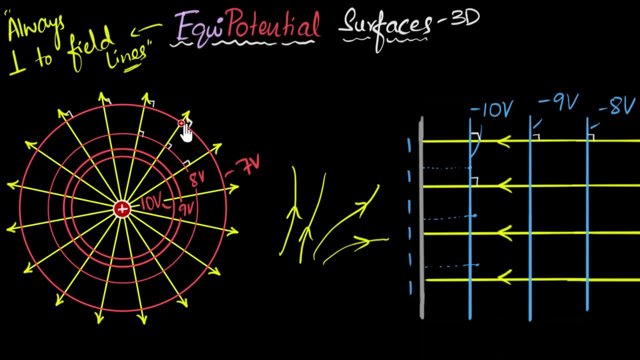 So here's my test charge. Now, imagine we move this charge along the equipotential surface, Say from here to here. Now, because it's an equipotential at every single point, the potential is the same. that means the potential energy of this test charge. 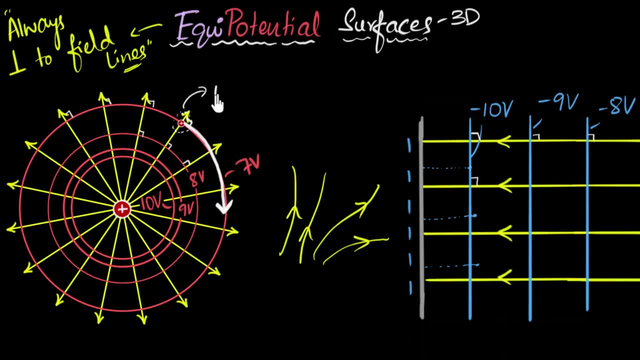 will remain the same as you move it Right. let me write that down: No change in potential energy as you move along the equipotential by definition right. No change in potential energy as you move along the equipotential by definition right. 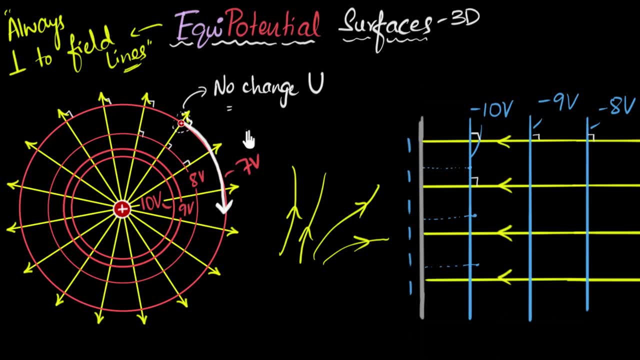 Okay, what does that mean? Well, if the potential energy is not changing, it automatically means no work done by the electric field, No work by the electric field. Now think about it for a second. Why should this be true? Because whenever electric field does work. 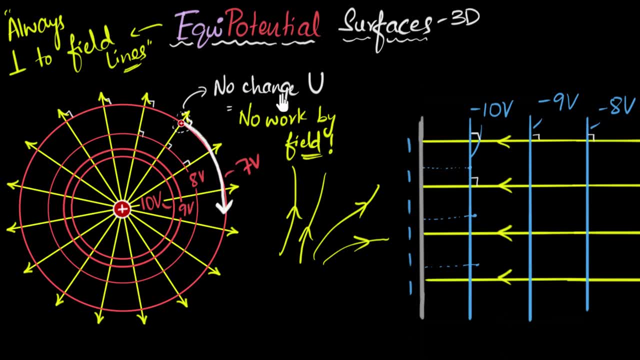 whether positive work or negative work, where automatically potential energy, where automatically potential energy would change. For example, let's bring back gravity, because gravity helps in understanding this. What happens when you drop a ball? Gravitational field does positive work. 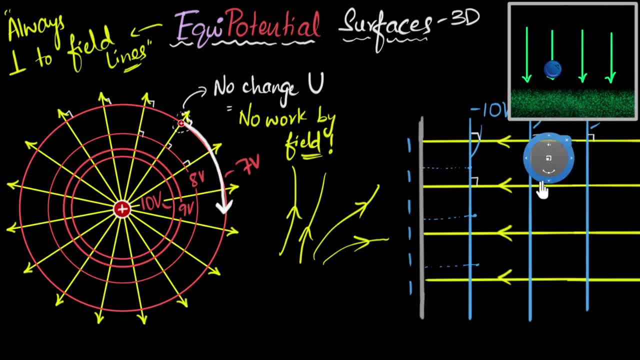 What happens to the potential energy? It loses it. What happens when you throw a ball up? Gravity does negative work. What happens to the potential energy? It gains it. So notice, whenever gravity does work, this ball would either lose or gain potential energy. 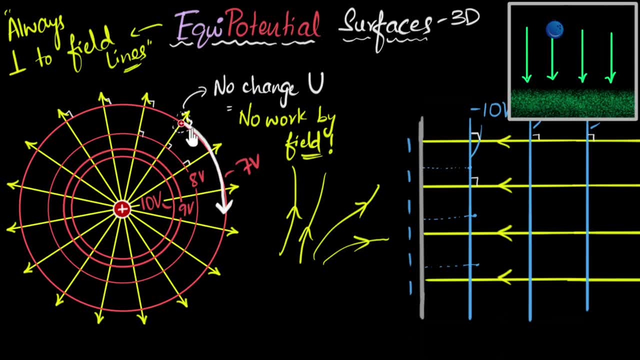 Same would be the case over here. If electric field did work, the charge would have gained or lost potential energy, But we are seeing that it is not changing its potential energy. Means that as you go from here to here, electric field must be doing zero work. 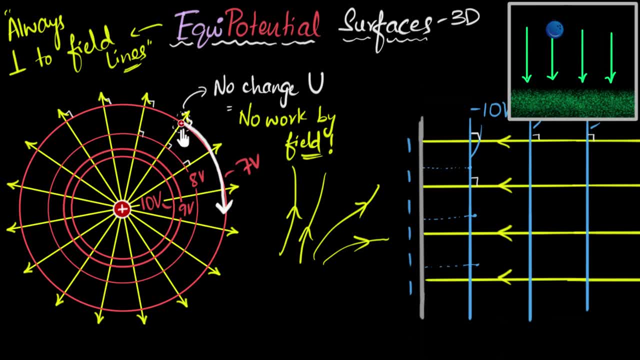 But how is that possible? Electric field is definitely pushing on the charges, putting a force on the charge, and the charge is moving. So how can work done be zero? Ooh, work done can only be zero if the force and the direction of motion are perpendicular to each other. 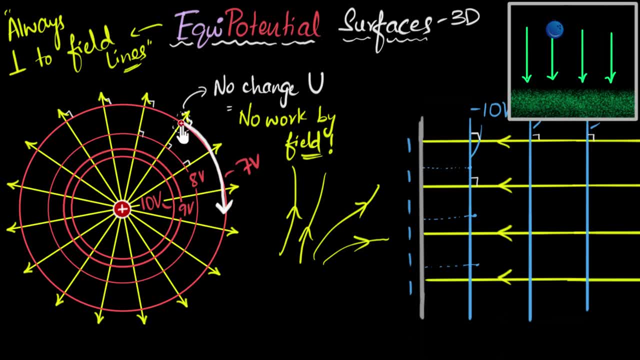 So, in short, as you move a test charge along the equipotential surface, its potential energy should not change. That can only happen if the electric field does no work, And that can only happen if, and only if, electric fields are perpendicular to the equipotential surfaces. 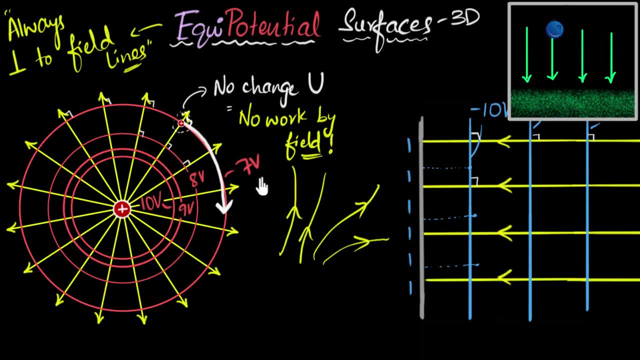 Now, if you find this a little hard to digest this right away, it's completely fine. It took me also a long time to do that. So keep pondering, keep thinking about it, It'll eventually make sense. So long story short, this basically means: 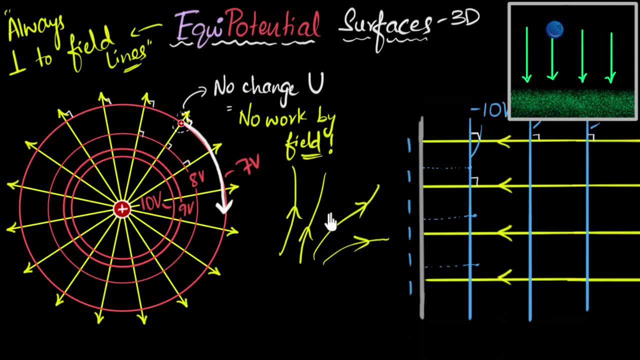 if you have been given some random field lines and if you want to draw equipotential surfaces, just start drawing perpendicular, drawing them perpendicular to the field lines. This is how you might do it And, of course, nobody's gonna ask you to do that.